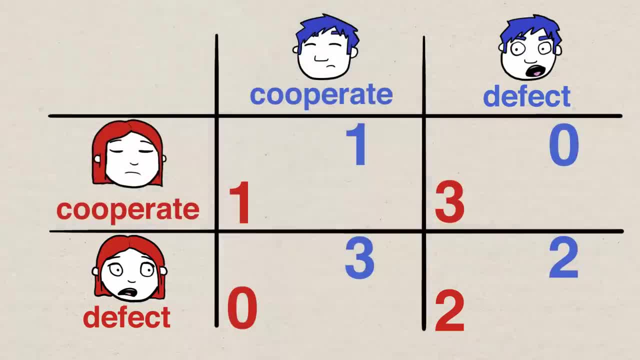 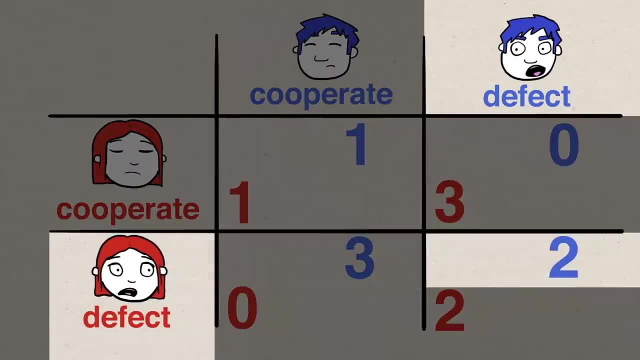 Two years in jail is better than three and being made a fool of Blue is in the exact same situation and will think the exact same thing. He should betray if she stays silent and he should betray if she betrays. They should have both cooperated. 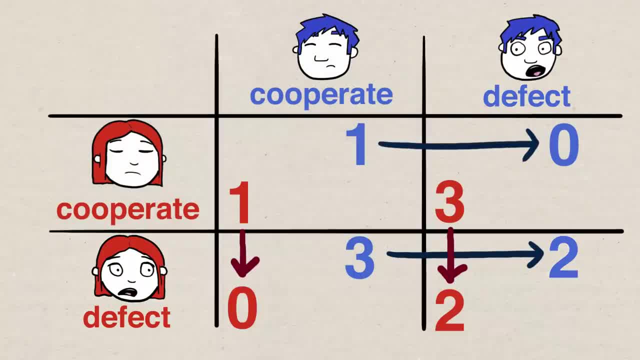 but from an individual standpoint they noticed they could always gain by defecting if they have no control over what the other person's gonna do. So they'll both defect to try to better their own situation, but come away not only hurting the group but themselves. 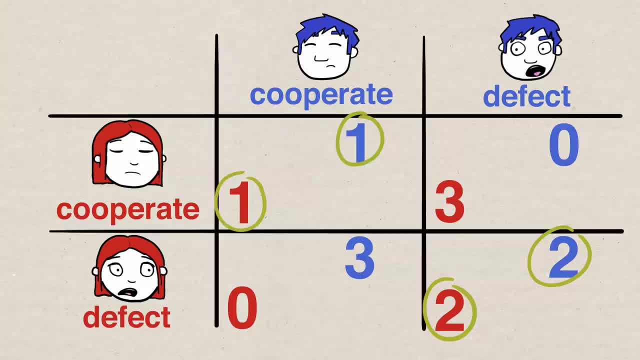 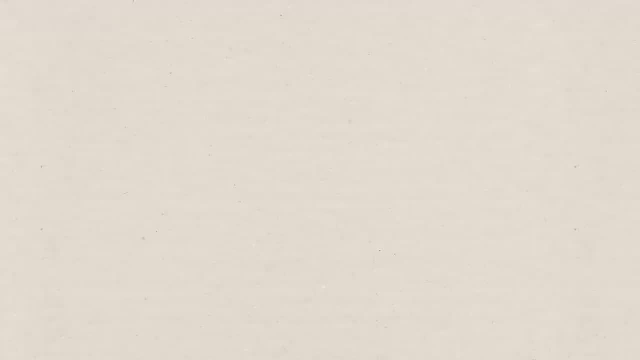 Individually they're worse off than if they both cooperated. This situation is pretty made up, but it has some real-world analogs. A common example is with marketing. Let's say two cigarette companies, Red Strikes and Smooth Blue. 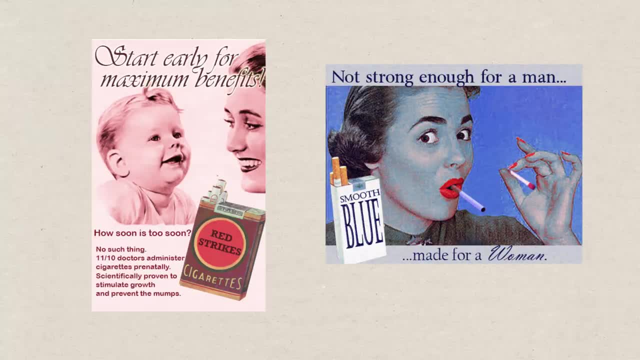 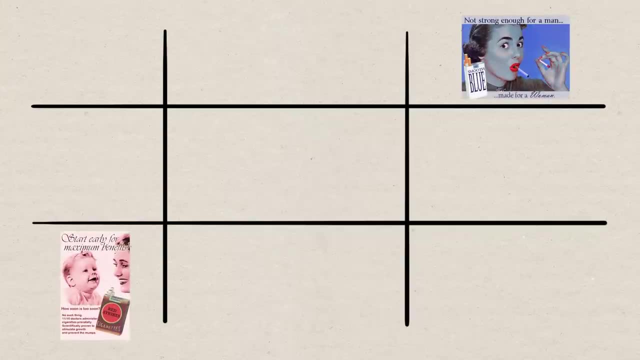 are deciding how much money they should spend on advertising. Since the product they each make is identical to one another, advertising has a huge impact on sales. For simplicity, let's say, their choices are to advertise a bunch or not advertise at all. And there's just 100 people in the society. 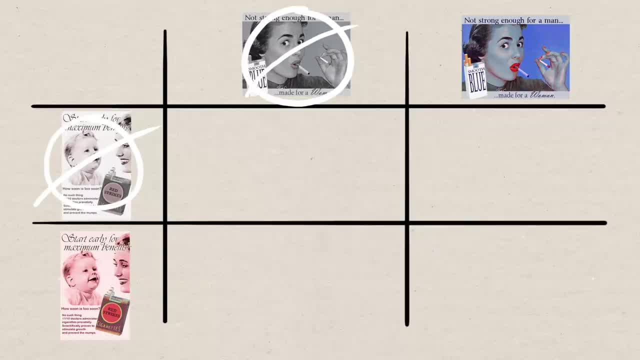 and they all smoke. If both don't advertise, then just by random chance picking cigarette boxes, 50 people buy Red Strikes and 50 people buy Smooth Blue. At $2 a pack they each make $100.. Let's say advertising costs $30.. 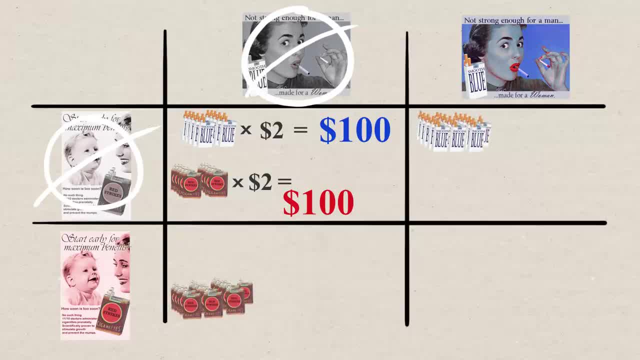 If one person advertises and the other does not, then 80 people will buy the cigarettes from the ads and 20 people buy the other ones. The advertiser makes $160 minus $30 for ads and comes away with $130.. The non-advertiser didn't spend any money. 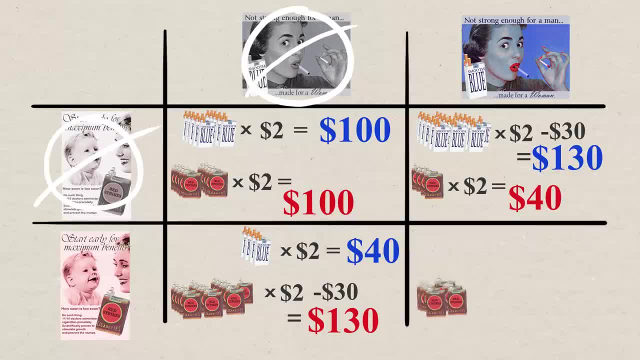 but only made $40.. If they both advertise again, half will buy Red Strikes and half will buy Smooth Blue, But since they both spent $30 on advertising, they only come away with $70 each. Same deal: Both people cooperating and not advertising. 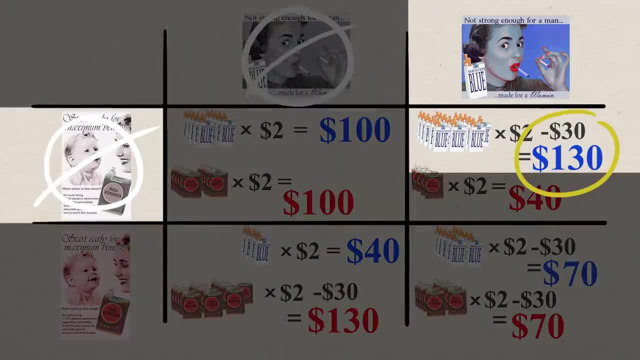 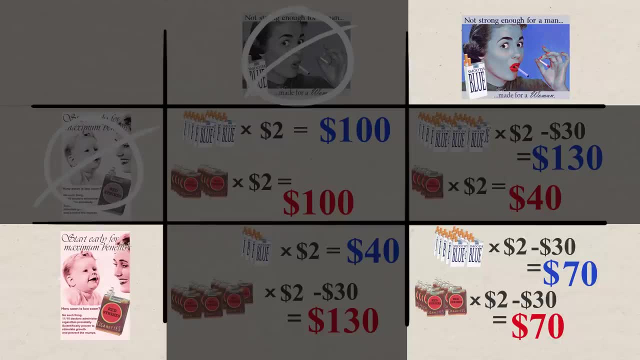 is the most preferable situation. but both companies can see that advertising will always make them more money. But unlike the prisoners in jail, these companies can talk and try to influence each other From here. Blue would be better off if Red didn't advertise. 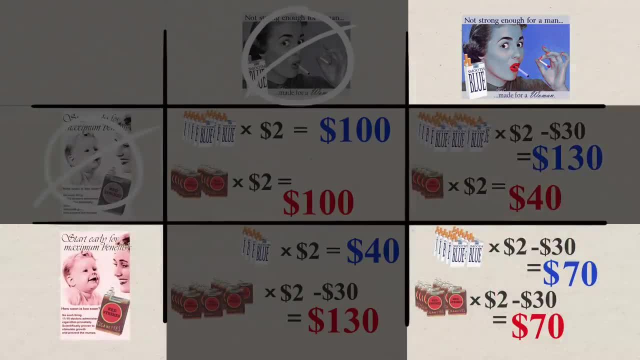 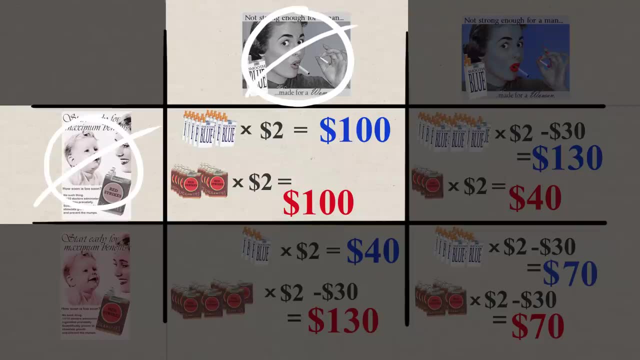 Red wouldn't go for that because that would be worse for them. Blue could try to convince Red that they would both not advertise the only other situation where they're both better off, But without any real obligation to each other. there's nothing that's stopping them. 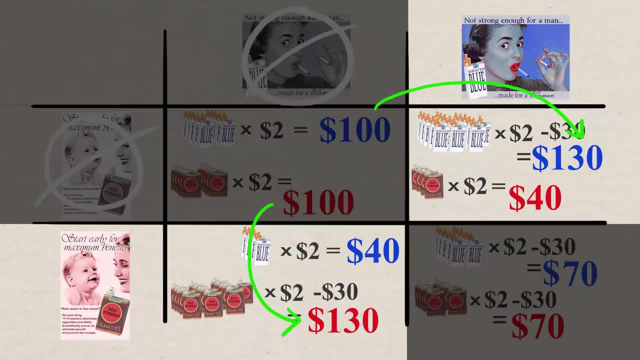 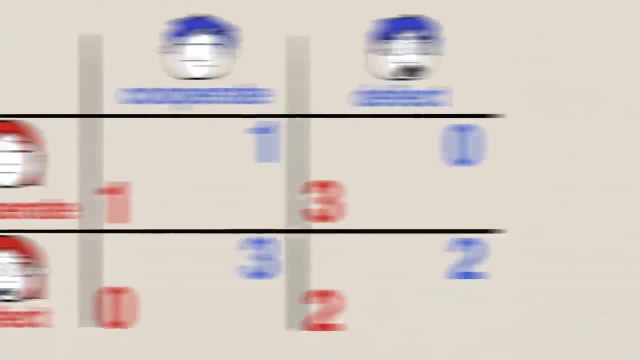 from trying to advertise to gain more of the market. anyway, If you think your opponent's gonna not advertise, then you're better off advertising, Although we're still making assumptions to make this situation work too. With this model, we're assuming they only play once. 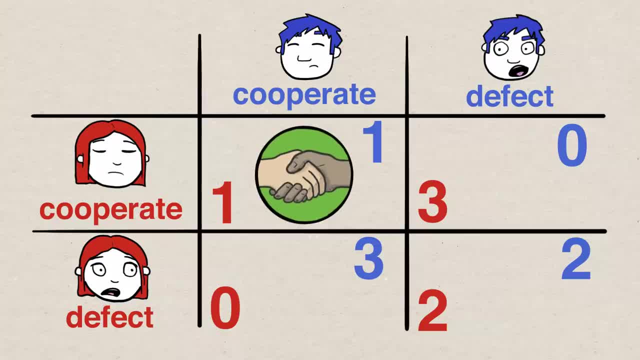 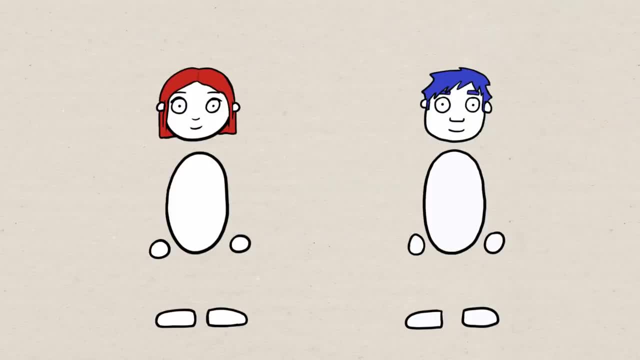 The game changes when the players have a chance to build a relationship and work together to get more gains over time or punish each other by not cooperating. Also, to make the model work, we have to make up rules for the players, Assume they're basically computer programs. 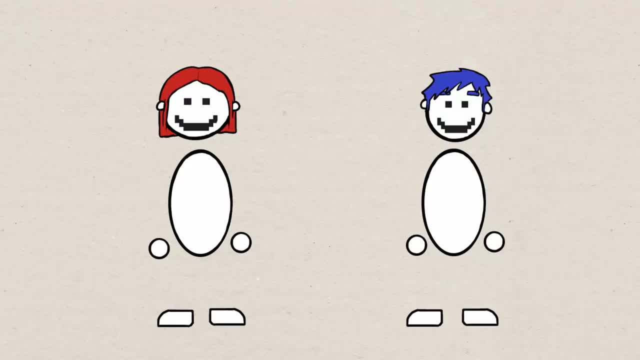 with predictable actions. These guys are creepier than they were in my head. They were supposed to be cute For the prisoner's dilemma and other similar models. we're assuming they are rational agents. A rational agent is a hypothetical person that will always pick the option that they predict. 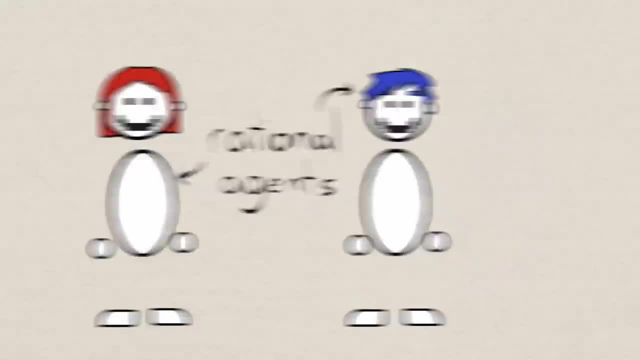 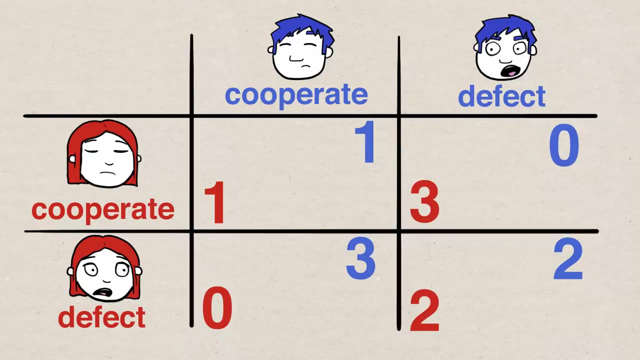 will work out best for them. They're not really thinking about the gains of someone else. Seems selfish, but it is something that real people generally do too. People always want what's best for themselves, and we don't like to be made a fool of. 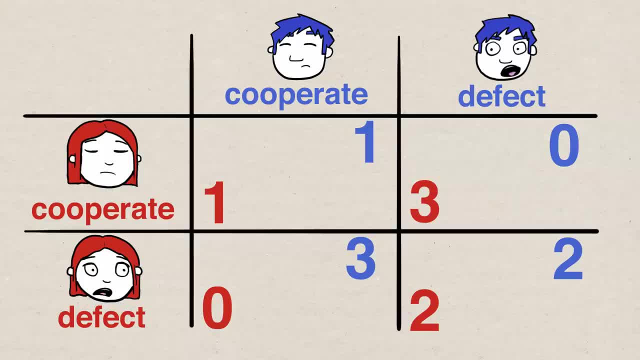 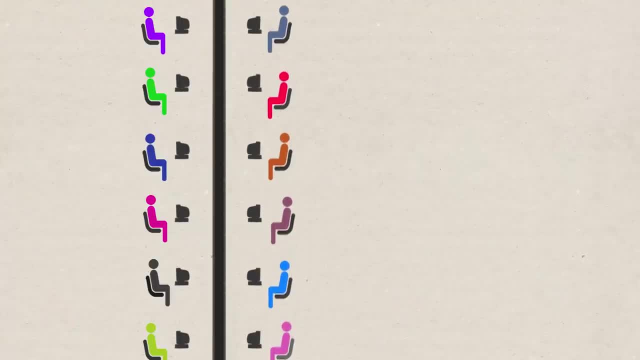 But if you put real people in the prisoner's dilemma, people don't always defect like the model predicts. In one study, 40 people playing prisoner's dilemma games through a computer without ever meeting or talking, only playing each opponent once. these are one-off games using a payoff matrix at least. 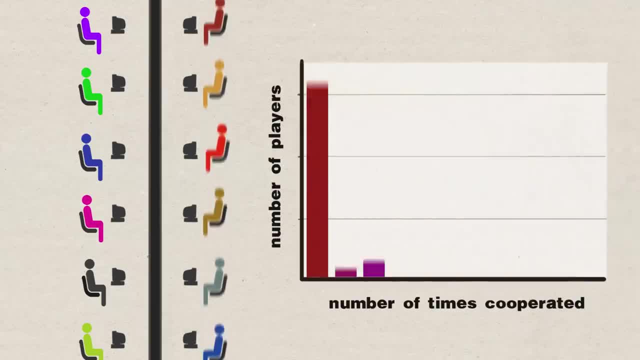 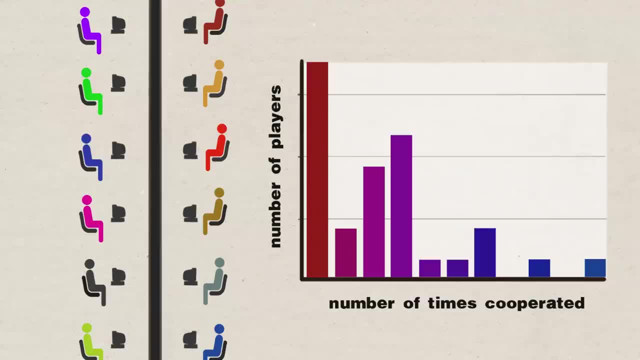 These guys cooperated on half of their games and everyone else is in between. This is a lot of cooperation coming from a model that predicts no cooperation. The largest group did act like rational agents, but most people tried to cooperate at least once. 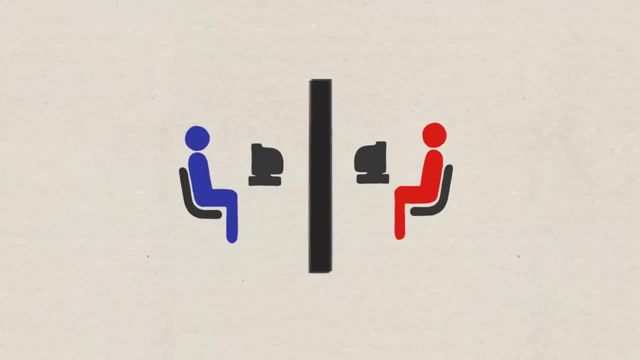 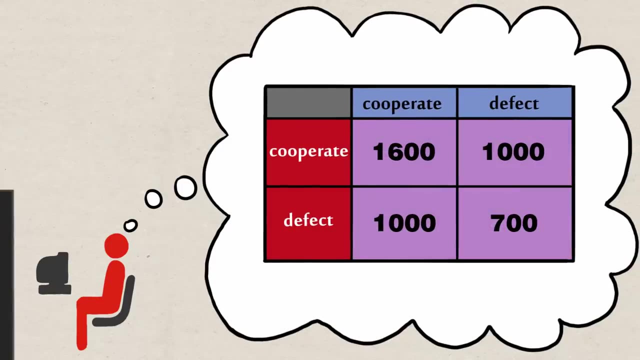 It's because, well, there's more to real people. We are social creatures and even in one-off scenarios with no guarantees or obligations and no chance to build a relationship, we're still thinking about how the group might decide. We're actually thinking from the perspective of the group. 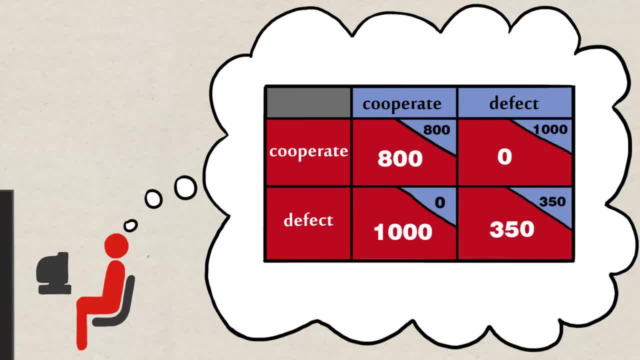 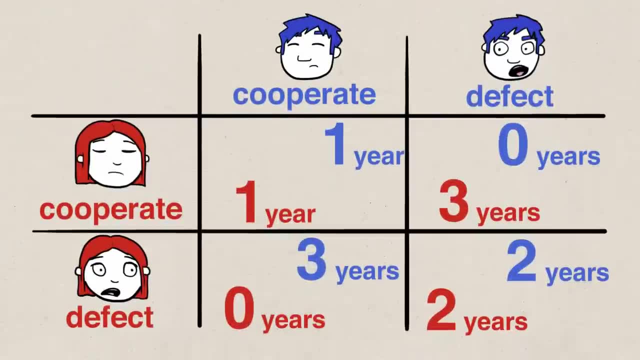 and making an optimistic decision. Cooperating an average of 20% of the time might not seem very optimistic, but remember this is with absolutely no communication or obligations. Anyways, that's not really the point. Using rational agents is still useful. 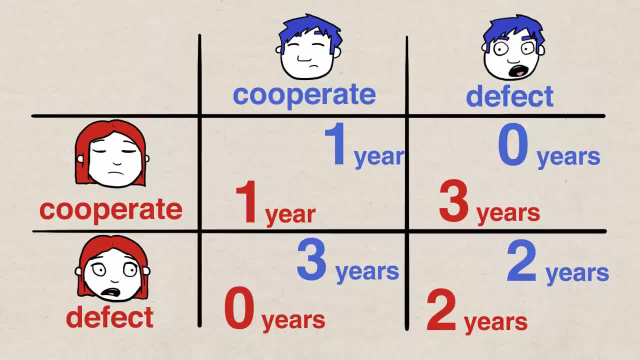 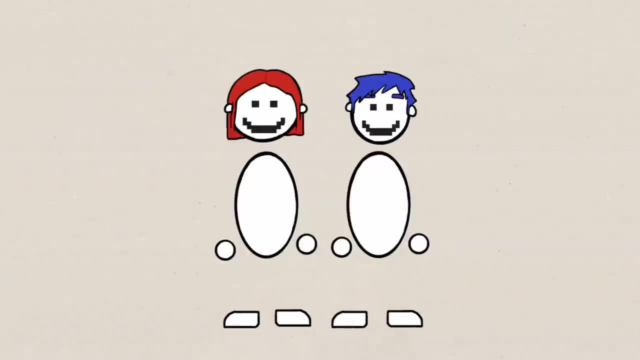 The model is just trying to point out the dilemma of certain situations where people are actually hurting themselves when, counterintuitively, they're only thinking about themselves. And that's why we're modeling using the cold, robotic psychopaths. You can be this weird being and say: